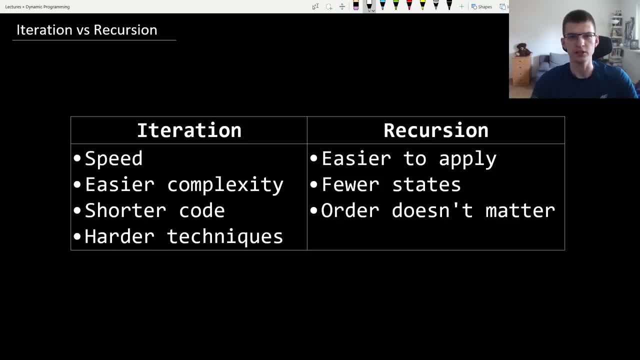 to approach dynamic programming. Iteration is usually about writing a few for loops that are nested inside each other. The advantages of this method are speed of a program. the overhead is smaller and thus the running time is smaller. Code is shorter and cleaner. 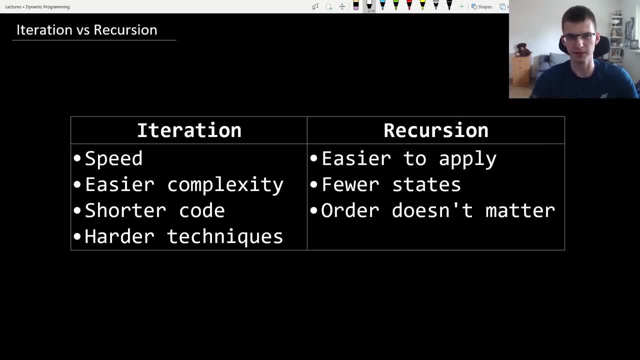 usually, and thus it's easier to say what is the time and space complexity of a program. And finally, in hard problems, sometimes iteration allows us to apply harder techniques like prefix sums and segment trees. On the other hand, recursion is easier because we can implement a naive solution or backtrack and then just add. 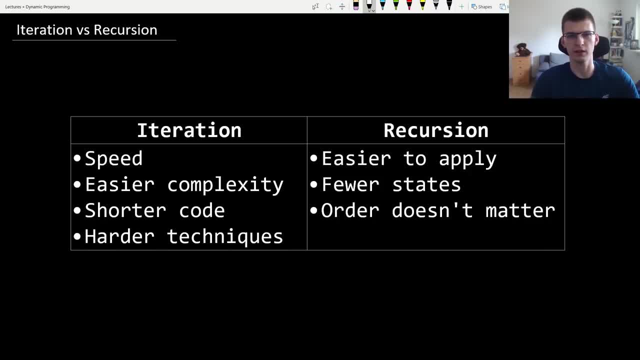 memoization, so it's easier to apply recursive dynamic programming to a problem. In some single problems, the number of states we will visit is smaller and the complexity might be even better, but that's not often the case. And finally, the order of states doesn't matter. 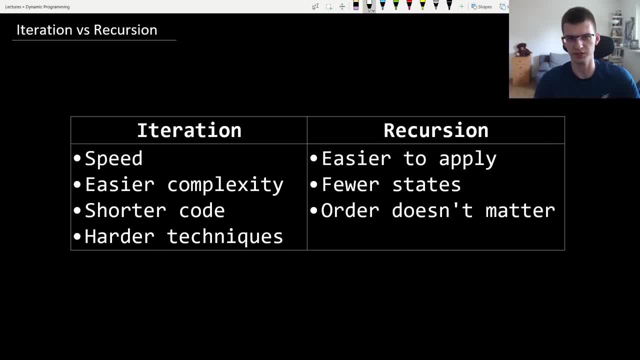 In recursion we don't have to care about the order of states, while in iteration we need to decide about it. It's hard, for example, in graphs: if we are given a DAG, we need to first apply topological sort to be able to run iteratively through vertices later and apply. 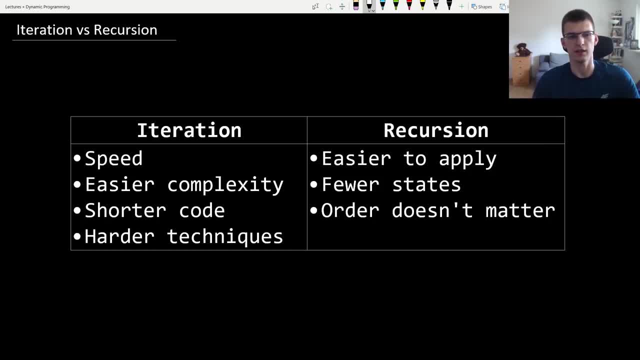 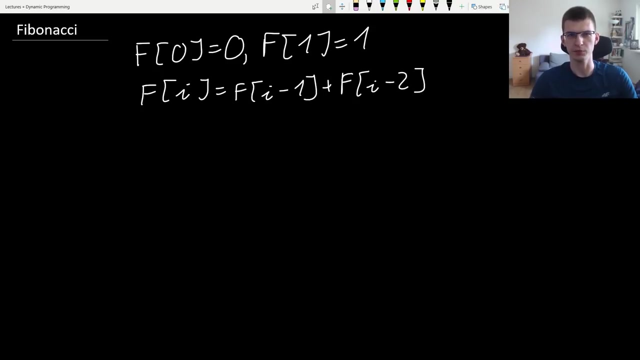 dynamic programming. That being said, especially because of smaller running time and being able to apply harder techniques, i strongly prefer iterative dynamic programming, and this is what most people do in competitive programming as well, among top participants. so let's stick with iterative. our first example is the fibonacci series, a sequence where the first two elements 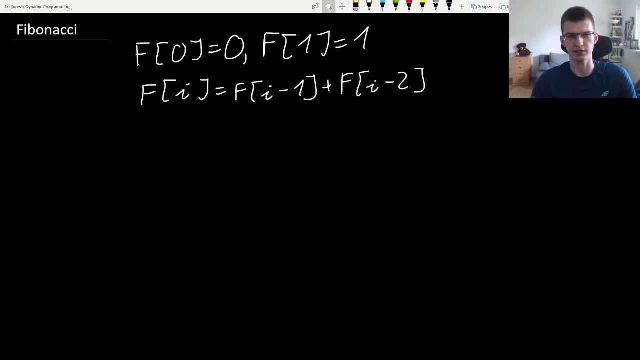 are 0 and 1, and then every next element is the sum of two previous elements. f of i is f of i minus 1 plus f of i minus 2.. we can implement a function that will recursively run itself f of given. i will sum up f of i minus 1 plus f of i minus 2, except for i equal to 0 or 1. then 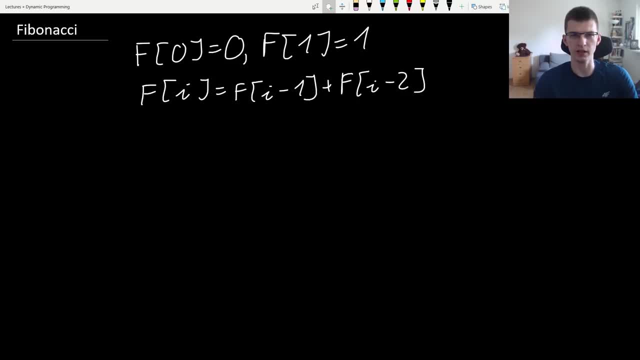 we know the answer immediately. if we run that for, let's say, f of 5 to compute the fifth fibonacci number, it will run f of 4 and 3, then f of 4 will run f of 3 and 2, and already we run f of 3 two times. some computations will be repeated unnecessarily. 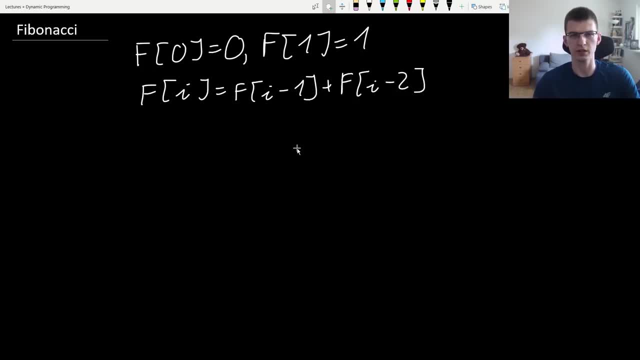 let's see the whole tree that shows us what are the calls. at the top we see the first run, f of 5, that needs f of 4 and f of 3 to be computed. then f of 4 runs f of 3 here and let's say: after all, the subtree is done, we have some value here, some x. 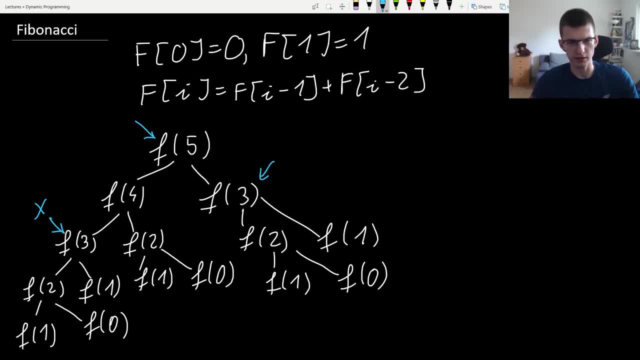 then much later, when we are on the right f of 3, we don't have to go below. this is what is called a repeated sub problem. we don't need to run that recursively. we just know that this is already that x, that we can save. same thing for f of 2, instead of computing that again running recursively if 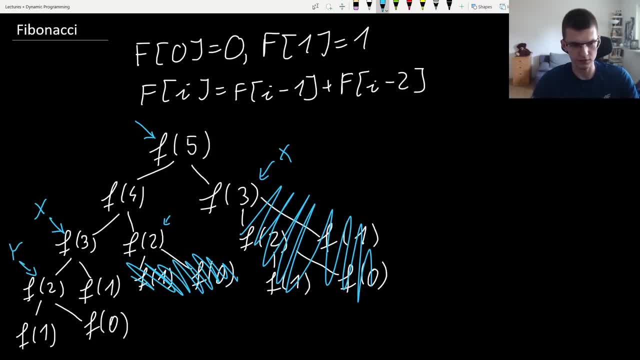 here we had a value y, then the same value should be here y. this way, our tree from the size, from exponential size, will become actually linear. let's see the implementation to make that more clear, now for a moment. you see the recursive solution with memoization added. if you want to, you can stop a video and read it. 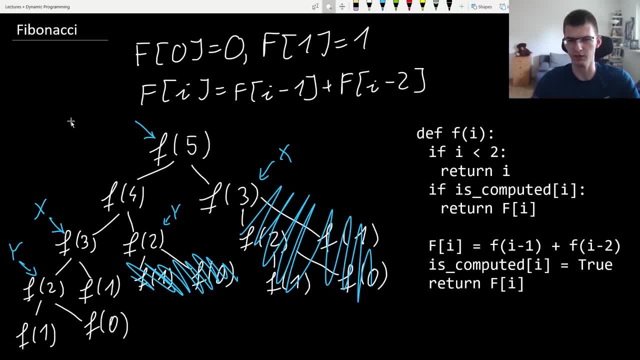 but we want to focus on the iterative version that is. here we create an array, f, we fill two first elements, f of 0 and 1- that's often called base case- and then we compute every next element using previous ones, because n fibonacci number needs values of n minus 2 and 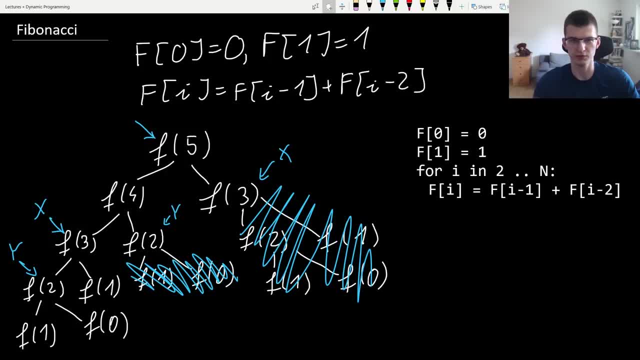 n minus first fibonacci numbers. those need previous numbers and so on. we anyway need to compute all the values up to n. this is why we just iterate through them and compute the values in constant time using 2 previous values. the order that we go from i equal to 2 to n is very important. 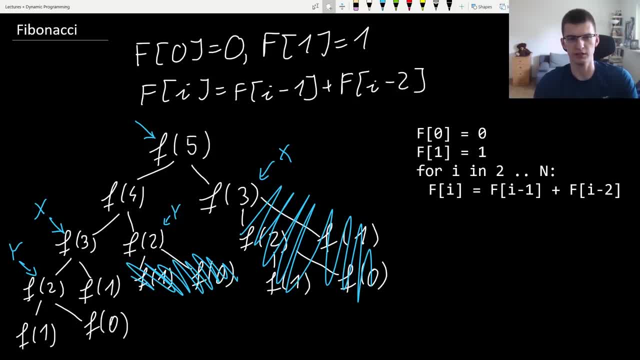 in iterative dynamic programming sometimes it's not that trivial. but once the order is chosen and some array, some state- here state is just i, f of i is the i fibonacci number, then we apply transition that somehow we get from the statement. this time, this time it was very interesting. 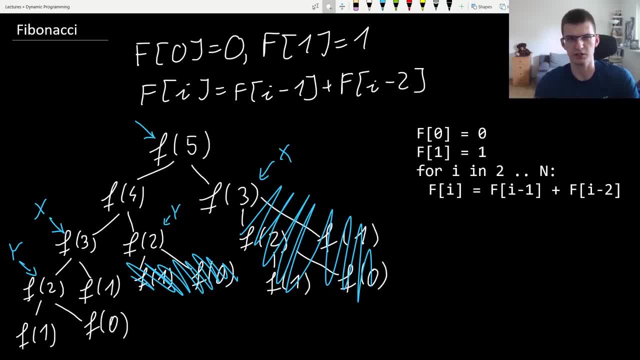 we can compute all like this easy because we were given a formula In next problems. it won't be that easy. Another bonus here is to solve the problem in constant time. If you have first and second Fibonacci number, you can use them to compute third one and 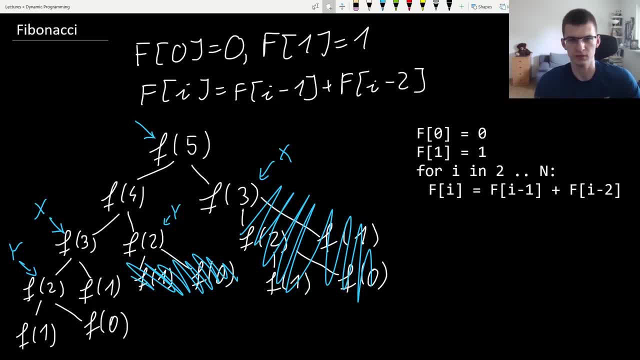 then you can forget about the first value. You can iterate and only remember the value of two consecutive Fibonacci numbers. use them to compute the next one and forget the i-th number and only move to i plus 1 and i plus 2.. This way, 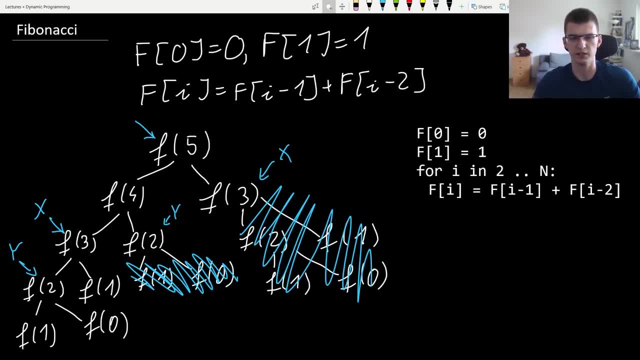 just with two variables and then choosing extra third variable, you can solve the problem in constant space. what is often a question in some contests or coding interviews, Let's see that dynamic programming isn't always necessary in those problems where we are given a formula. One example of that is a. factorial. Factorial is a function that is used to calculate the number of variables in a given space. Factorial is a function that is used to calculate the number of variables in a given space. Factorial is a function that is used to calculate the number of variables in a given space. 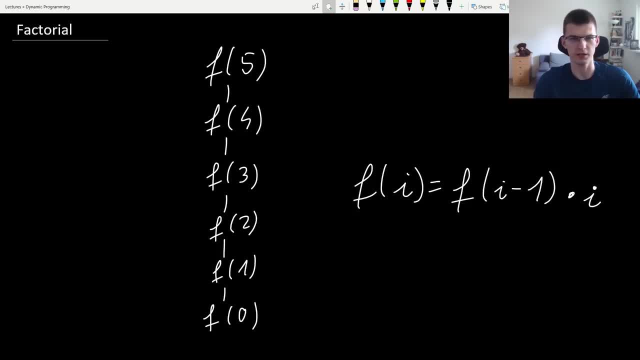 Factorial of i is defined as factorial of i minus 1 times i. If you draw a tree that shows what recursive function will call f of 5, will call f of 4 and so on. there isn't any repeated work and this means that dynamic programming isn't. 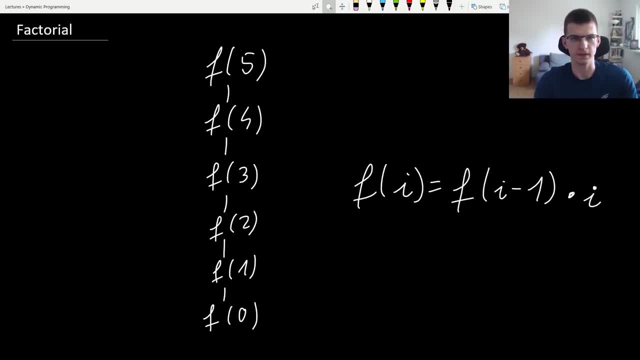 necessary. Still, you can create an array and f of i you can compute as f of i minus 1 times i. It's actually useful if you want to remember all the factorials and then be able to answer for the i factorial in constant time. but if you just want to compute one, then a for loop. 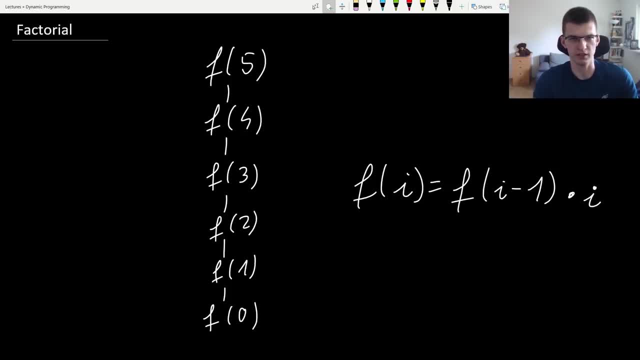 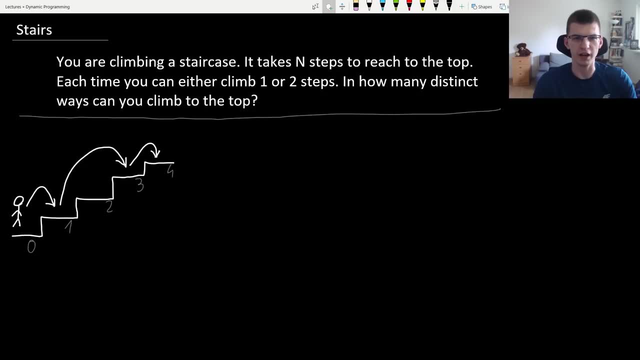 is enough, or a recursive function- both will be just linear and DP isn't necessary. There are two examples left, and in them I will show you how I think about a dynamic programming problem and how I approach choosing a state and transitions. First problem state: 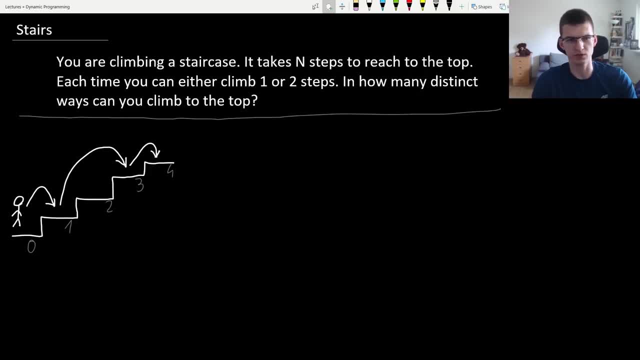 If I want to go to the top of the pyramid, I have to do this step by step. In this case, you can do it like this: We will take a step in the pyramid and we will count it like this. Next step is to climb the stairs. You're climbing stairs. it takes n steps to reach. 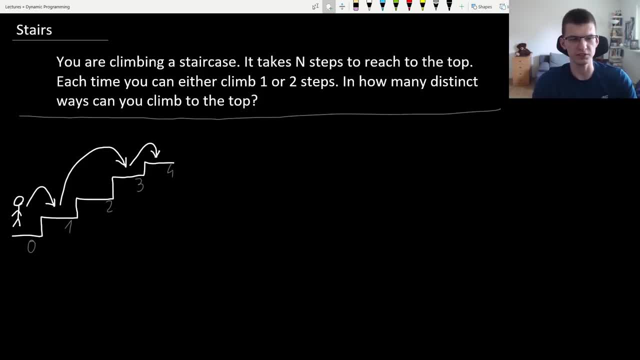 to the top. each time you can either climb one or two steps, Count distinct ways you can climb to the top and there's an example with four steps to climb and one. answer modulo some value, otherwise it would be huge. when we are at some step, let's say here: 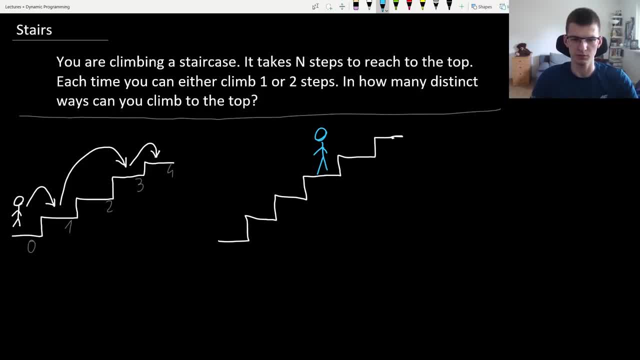 it doesn't matter how we got here. maybe we took single steps, maybe it was first two steps, then one step. it doesn't matter, because the problem doesn't tell us, for example, that two consecutive steps can't be of size two, something like that. it only matters where we are. this is why. 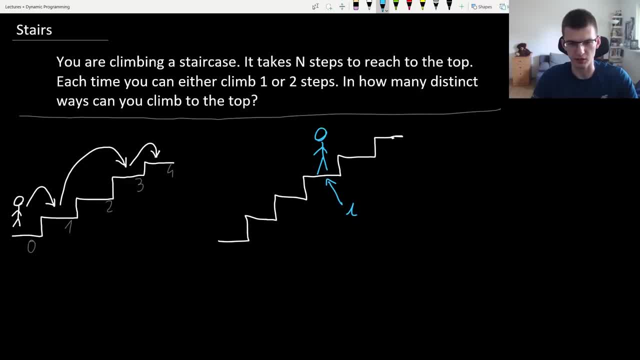 the state must be just a position. i or pos like position, and this suggests the dimension of dp should be that i position. because the problem tells us to count ways, i will define that as integer int dp of i. that means the number of ways to get here. 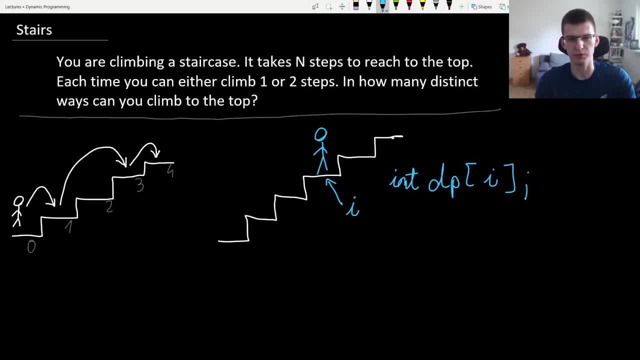 if the problem asked me to compute the minimum number of jumps to make something, then that would be the minimum number of jumps. if the problem asked me: is it possible, then this would be just a boolean value that says whether I can get here. yes or no, true or false. if we need to maximize something, that would be maximum value. 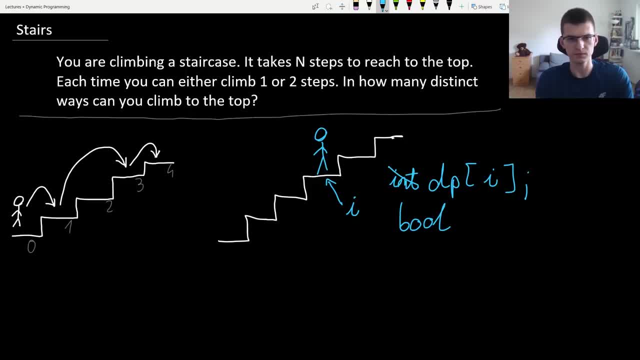 that we need to maximize to get here. if we define the state as int, dp of i, the number of ways to get here, then we have an easy transition because we know to i we can get to i minus, from i minus 1 or i minus 2, then the transition is dp of i. 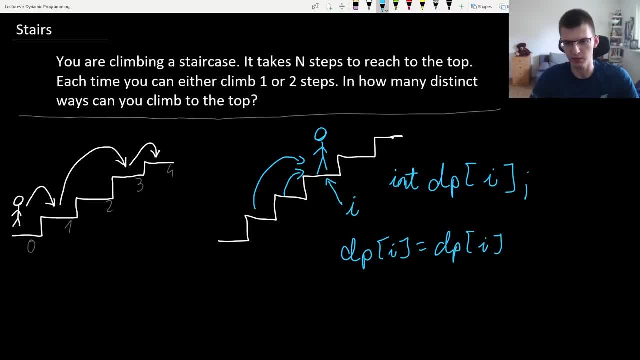 is dp of i minus 1 plus dp of i minus 2. you can see here similarity to the fibonacci sequence and actually is the same thing it's. the story is different, but the problem is exactly the same and the answer will be the same. maybe to any you should add or subtract one, because the base case might. 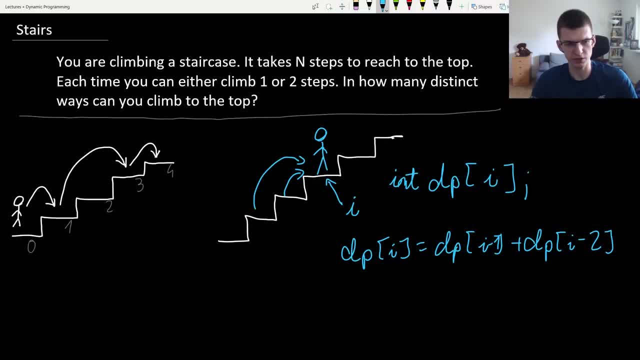 be different here. the number of ways to get to 0 step is one. this is just an empty path. then to the next one is one and every next step. the number of ways is the sum of two previous values. Here the answer would be 5.. But what if the 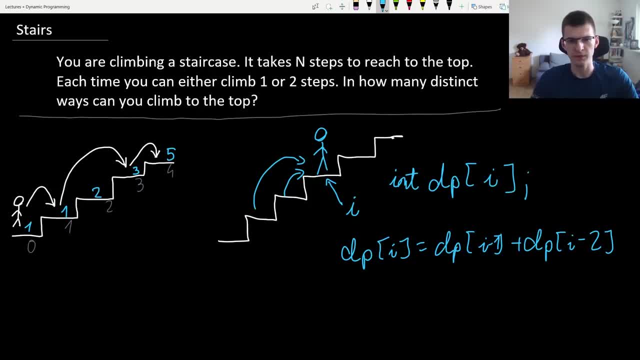 problem is more complicated. What if we're additionally added? we are given value k and the statement said: at most k jumps or well moves you make At most sorry, at most k jumps. Then when you are at some position, i, you can't anymore. 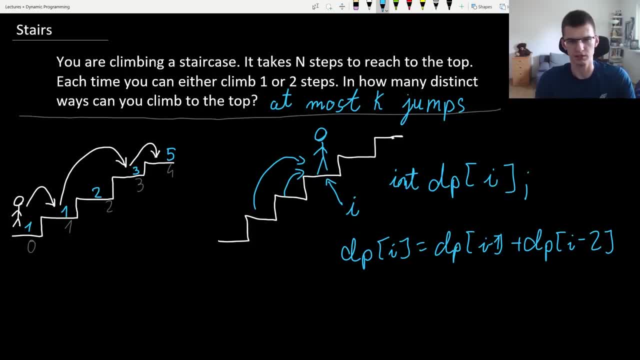 say it doesn't matter how you got here. There are exponentially many ways you got here, but what is important is the number of jumps you made. There is a difference, if you are here, whether you made one jump, two or three or maybe zero, if that's possible. 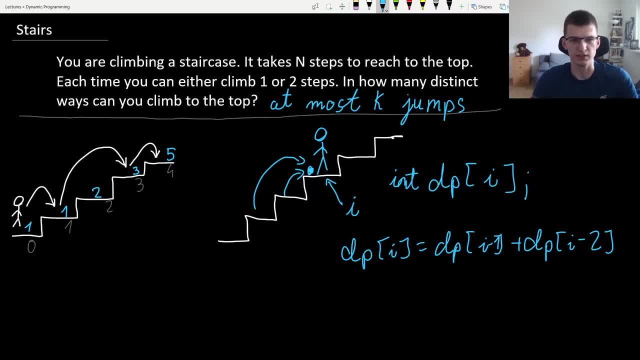 This means we should add that as a dimension of dp The state isn't just described as position, it's also the number of jumps to get here. Then I change that to dp and let's say lowercase k. that means the number of jumps to that position At the end, instead of just printing dp, the. 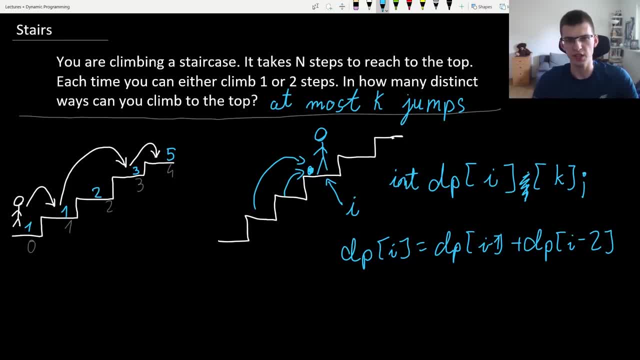 number of ways to get to the nth step. we'll print the sum over. the answer will be the sum over dp and j, the number of jumps over j from 0 up to k, because we are allowed to make at most k jumps. It's easy after that define to see. 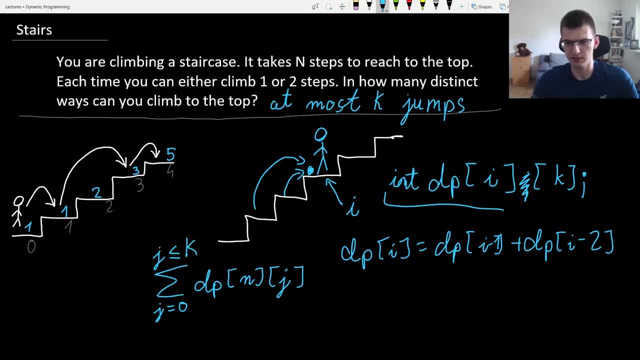 the complexity, as well The space complexities, O of times, k given in the input. Those are two dimensions and every state you compute in constant time. dp of i, k is dp of i minus 1 or minus 2 of k minus 1.. To that: 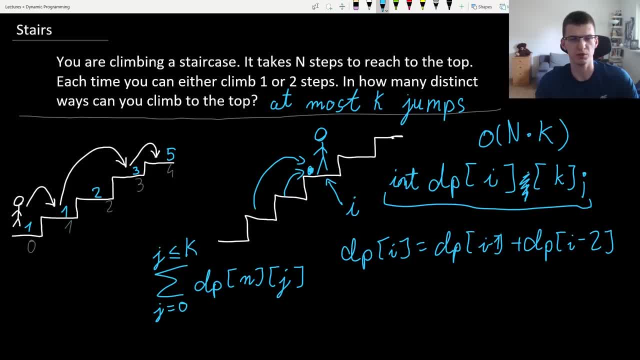 previous step, you made the number of jumps smaller by 1, and this is exactly how I approach dynamic programming problems. I think when we are at some position, what is important so far Is the number of jumps is important. Maybe the last jump is important because we are forbidden to make two same consecutive. 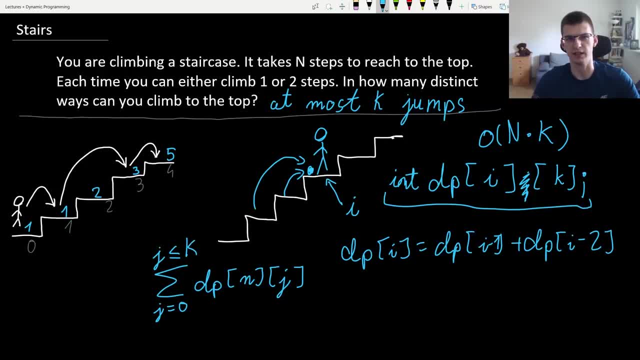 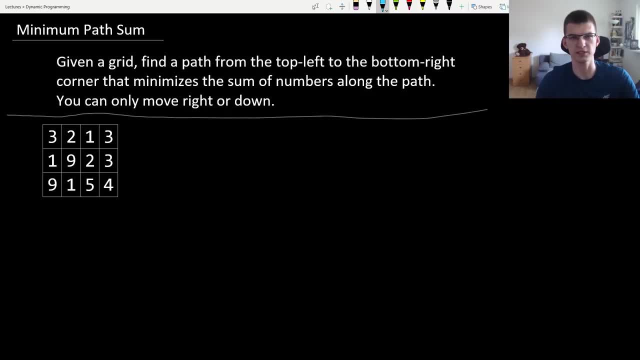 jumps. Let's see the same thing on the next problem: Minimum path sum. Given a grid, find a path from the top left to the bottom right corner that minimizes the sum of numbers along the path. You can only move right or down each time. 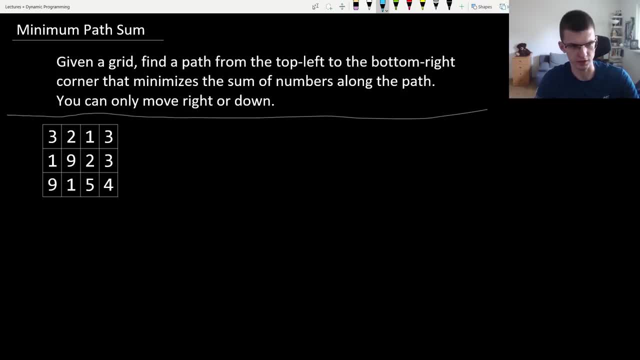 For example, given this grid with 3 in the top left corner, from the bottom right corner to the bottom left corner, you can only move right or down each time. For example, given this grid with 3 in the top left corner to the bottom right corner, you can only move. 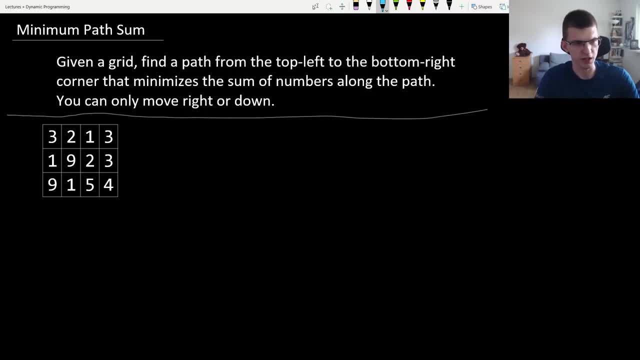 from which we should start. The optimal path turns out 3, 2, 1, 2, 3, 4.. Remember that we said, for problems that ask you to optimize some value, not count the number of ways, you should often think about an easier greedy approach Here. 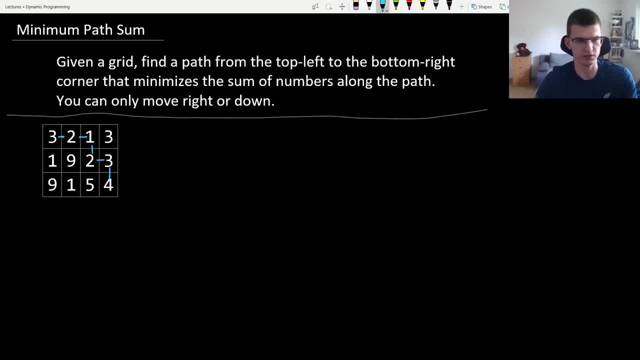 that idea would be to maybe go to that neighbor of yours, starting, let's say, from 3,, that is, smaller, From 3, maybe greedily we should take to 1, but this example already shows us that it's a bad approach because maybe in a moment we'll have to get to a big number here, a 9.. 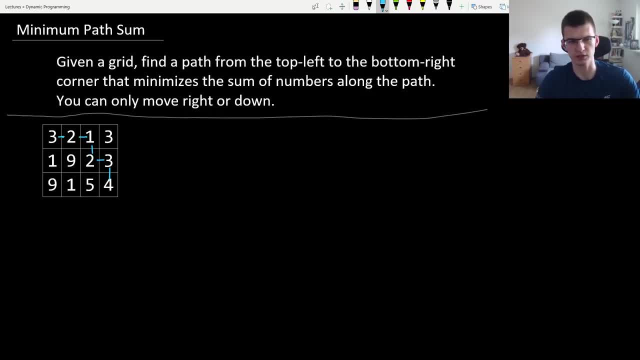 And if greedy doesn't work, then usually dynamic programming is a way to go. We will try the same approach that I told you about for the previous problem. When you're at some position, actually sometimes you can think about it after some time after. 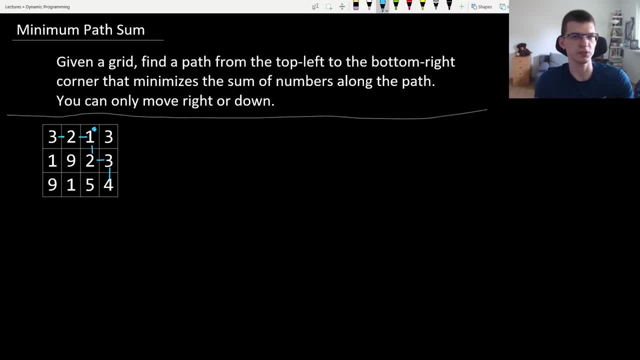 some number of steps or seconds. what is important so far? When you are, let's say, at this 2,, it doesn't matter whether you visited maybe this 1.. It doesn't matter what exactly is your path other than the score so far, the sum of values Here. it. 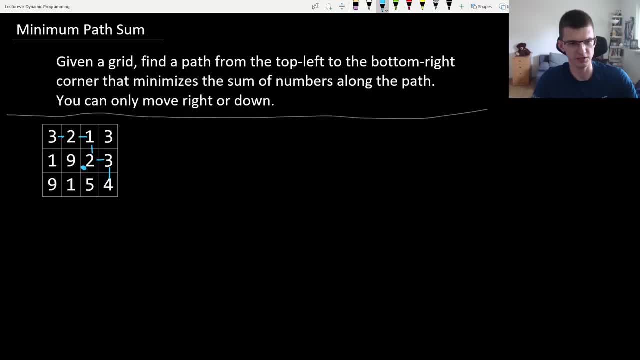 would be 3,, 2,, 1, and 2, and this is why I would say dp of that row and column, because this is the is. in that case, it would be what 538 int dp of row call is the minimum sum so far. minimum because the problem asked us to minimize that sum of numbers. 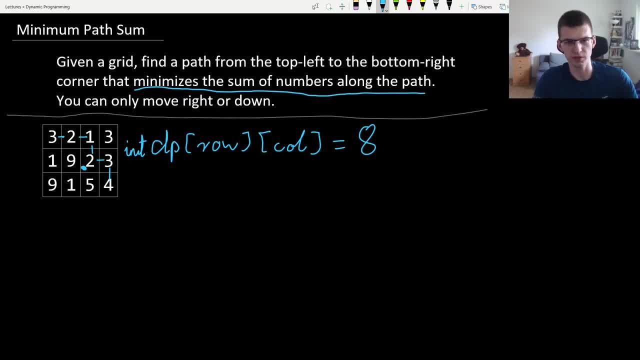 along the path: minimum sum of numbers so far up to this moment. and yet we will just print this value dp in that position as the answer. as with previous problems, transitions are very easy because when you are at some cell row call, you know that previously you had to be in one of one of cells to the left. 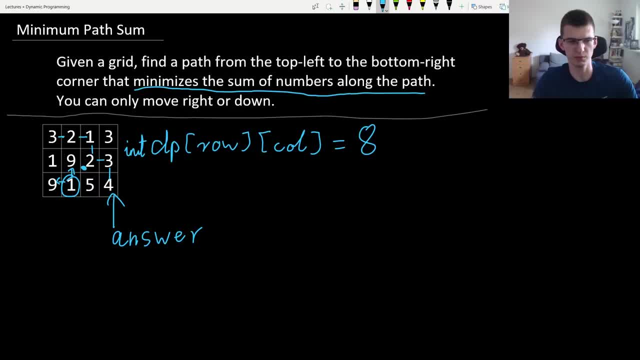 or to the top. you need to take the maximum of those values, dp plus the value in this new cell, because you extend a path by one. if this problem told you, for example, that you cannot make two consecutive steps down, then you can't anymore. say the only thing that matters. 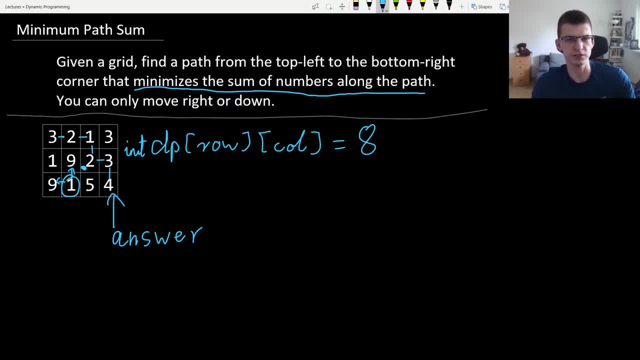 so far is the sum of values but also the previous step. so for a problem where you can't make two consecutive steps down that dp would be row column and here 0 or 1 for dp or the previous step, whether it was right or down, if that previous step is. 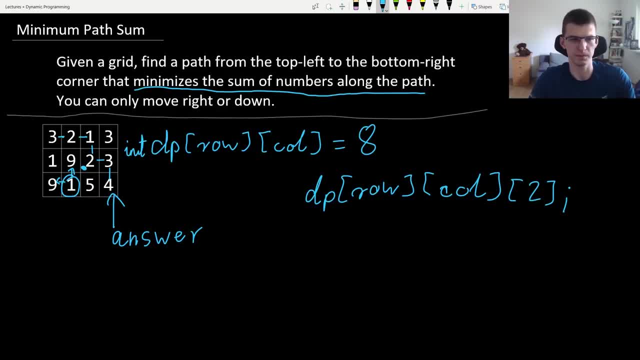 down, then the new one can't be. one more thing that we'll talk for future lectures is forward versus pull from previous dp. here dp of row call we can compute as the maximum of two previous numbers, or alternatively we could use already computed dp of row call for some. 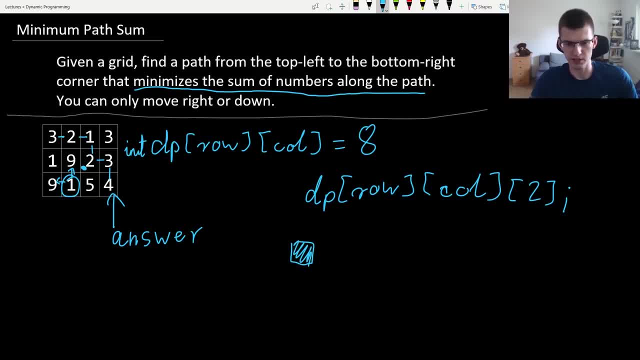 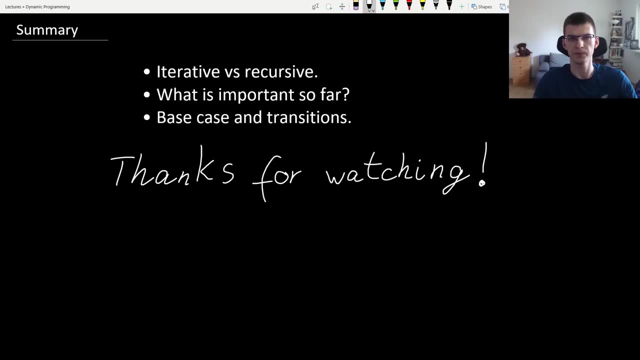 number, and later we would use that variable dp, 아마 in the top, then plus the value from that of rows 0 to the top excess, and then you can take the conversation between one cell's value and that less than the result and calculate it that this improvement is. 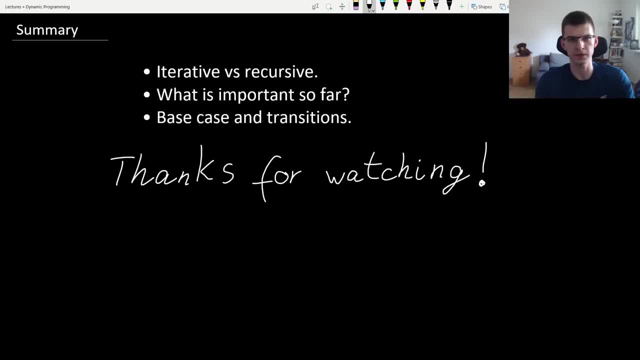 effective because you can search current, para��, current trend and future trends directly, so to say, when we are at some position. what is important to remember so far? not exactly the shape of a path that we went till this position, but the sum of elements that we 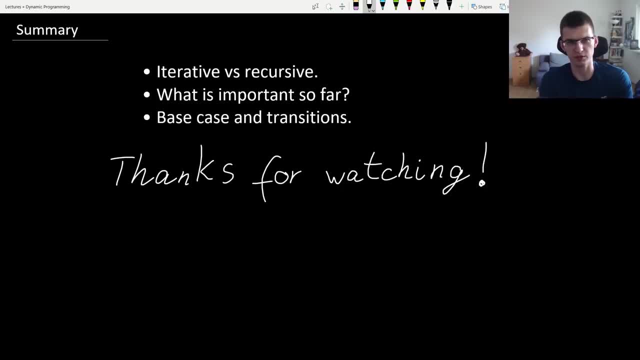 need to minimize or the last step or the number of steps that is required to move forward, because the problem tells us some limit for the number of steps. Finally, you can go through problems we talked about and make sure you understand what base case to put there. so how to initialize the array if you want to minimize something and 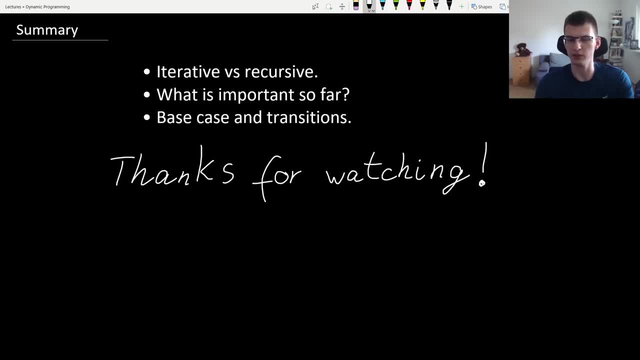 you need to fill all the values in the array, then maybe infinity is a good idea and just put zero in the very first cell. Otherwise, if zeros are everywhere and you need to minimize something, there will be still minima everywhere, Plus transitions. usually come from the statement. 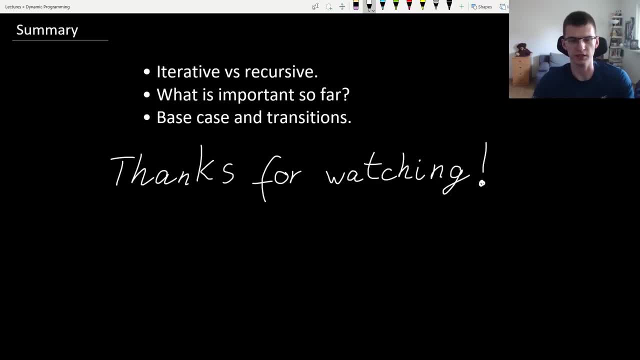 In those problems that we talked about it was quite easy to see that to some cell you can get from to neighboring cell, to previous cells. In the next lecture we'll see obviously harder examples And finally, either in the next lecture or in some videos, I will again go through AddCoder. 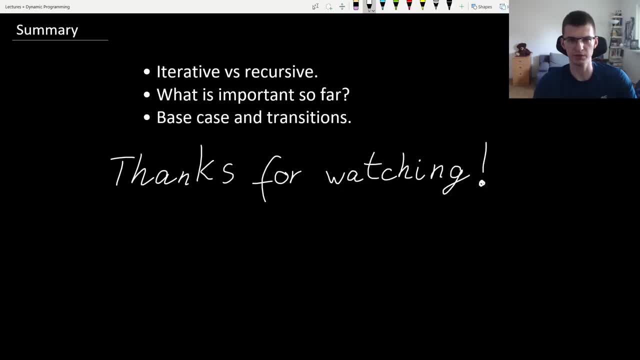 dynamic programming contest problems, at least first six problems, and there we'll apply multiple, not-so-easy techniques. Right now, I want to thank you for watching and see you in the next dynamic programming lecture. Bye, bye.